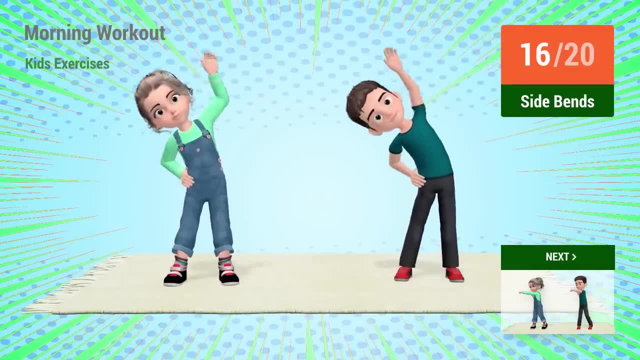 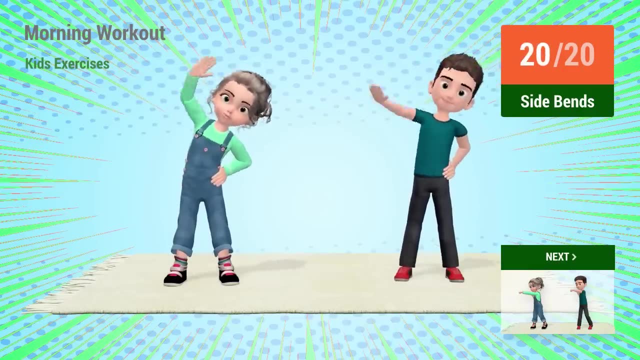 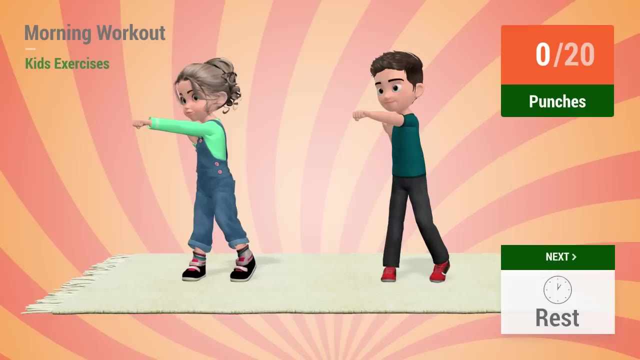 16,, 17,, 18,, 19,, 20.. Up next punches in 5,, 4,, 3,, 2,, 1.. Go 1,, 2,, 3,, 4,, 5,, 6,, 7,, 8,, 9,, 10,, 11,, 12,, 13,, 14,, 15,, 16,, 17,, 18,, 19,, 20.. 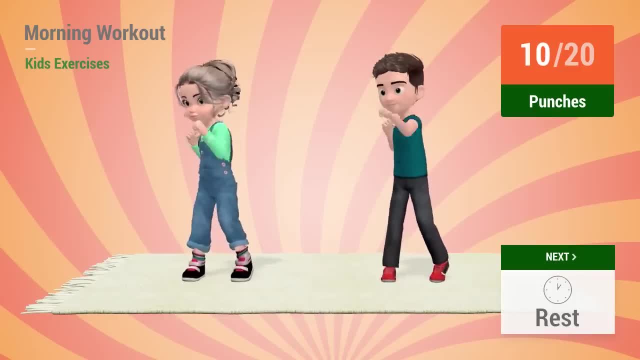 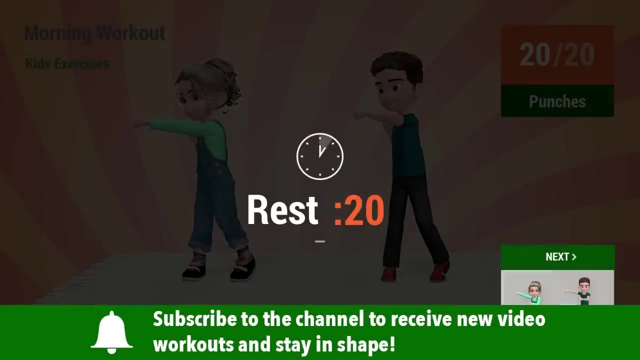 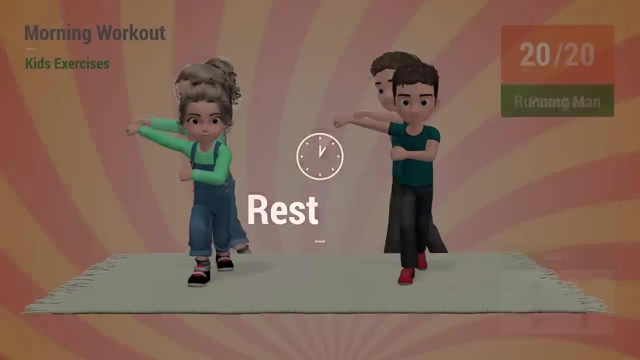 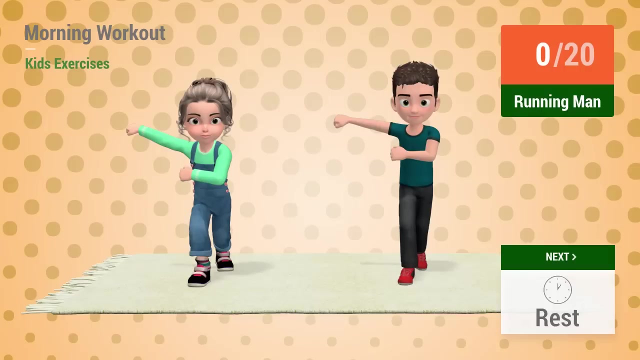 8,, 9,, 10,, 11,, 12,, 13,, 14,, 15,, 16,, 17,, 18,, 19,, 20.. Rest time Up next running man in 5,, 4,, 3,, 2,, 1. Go. 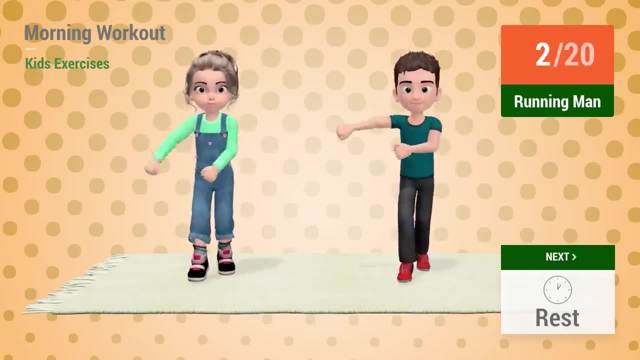 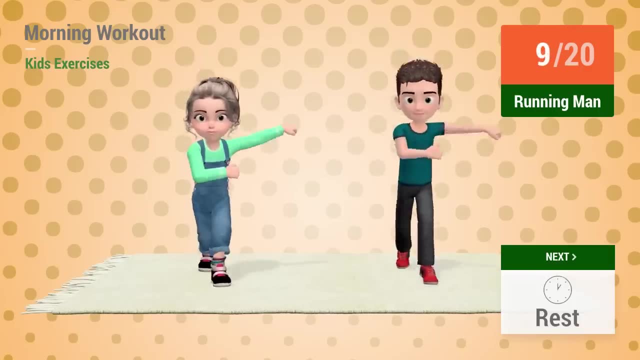 1,, 2,, 3,, 4,, 5,, 6,, 7,, 8,, 9,, 10,, 11,, 12,, 13,, 14,, 15,, 16,, 17,, 18,, 19, 20.. 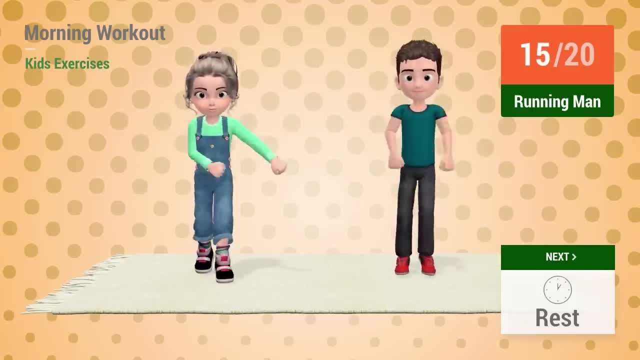 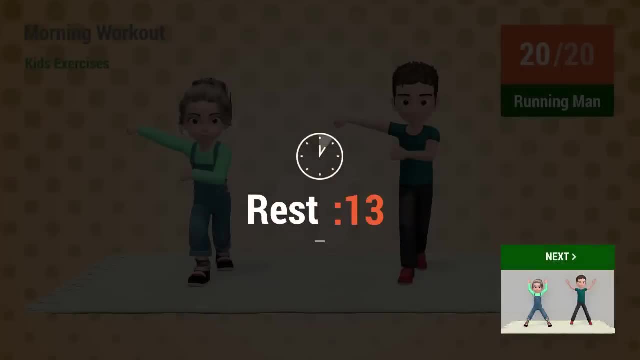 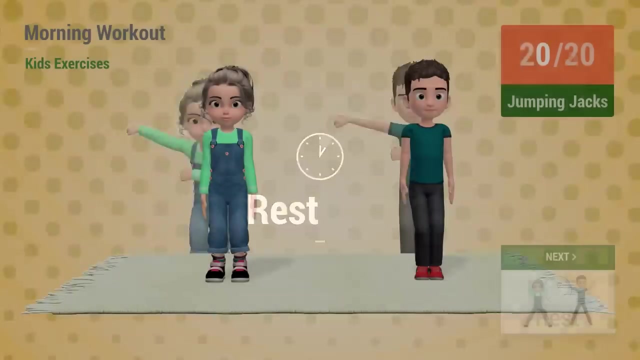 Rest time. Up next jumping jacks in 5,, 4,, 3,, 2,, 1.. Go 2,, 2,, 3,, 4,, 5,, 6,, 7,, 8,, 9,, 10,, 11,, 12,, 13,, 14,, 15,, 16,, 17,, 18,, 19, 20.. 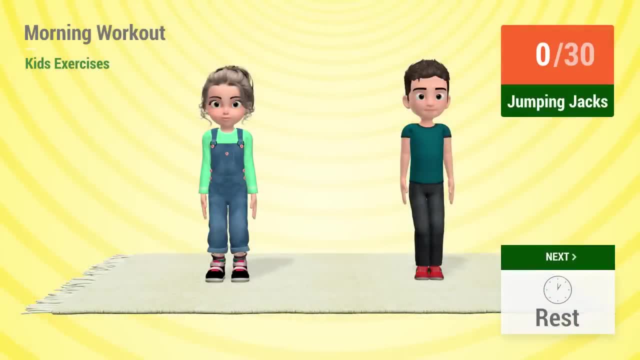 Rest time. Up next jumping jacks in 5,, 4,, 3,, 2,, 1.. Go 1,, 2,, 3,, 4,, 5,, 6,, 7,, 10,, 11,, 12,, 13,, 14,, 15,, 16,, 17,, 18,, 19,, 20.. 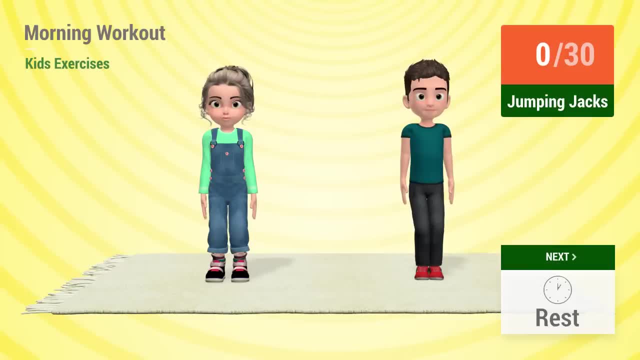 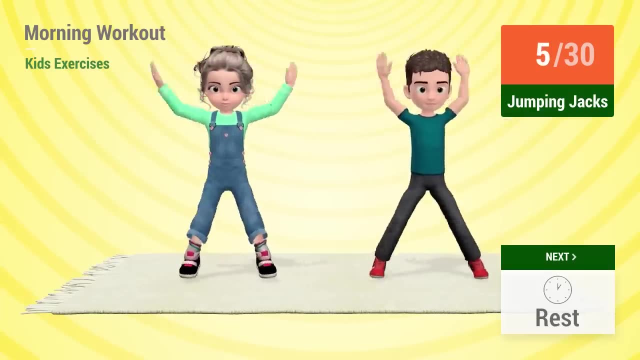 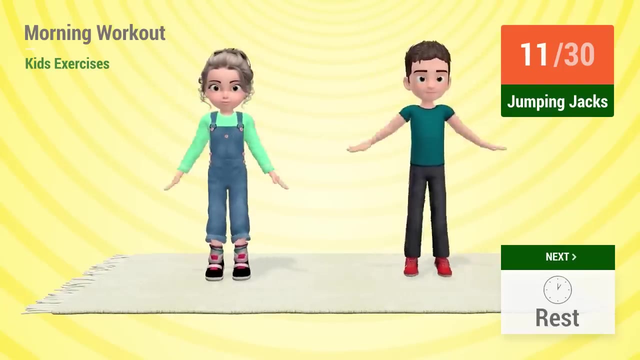 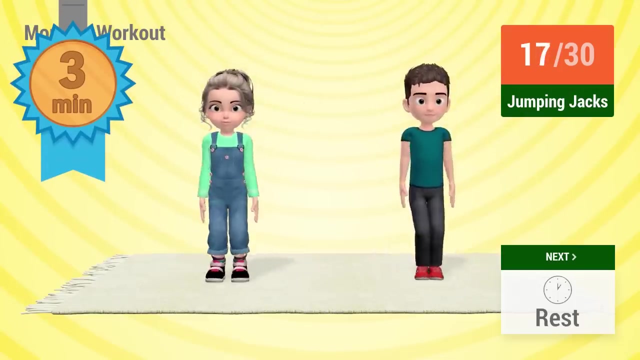 Rest time 3, 2, 1, go 1, 2,, 3,, 4,, 5,, 6, 7,, 8,, 9,, 10,, 11,, 12,, 13,, 14,, 15, 16.. Congratulations, You've. 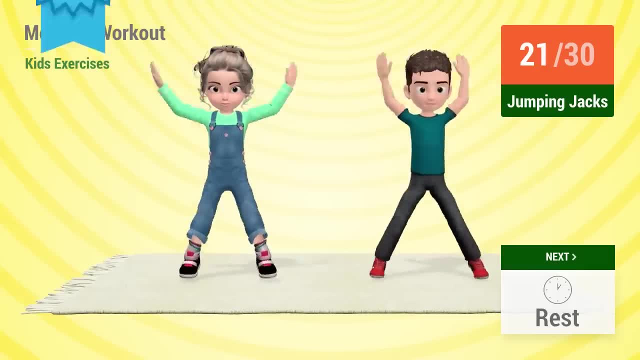 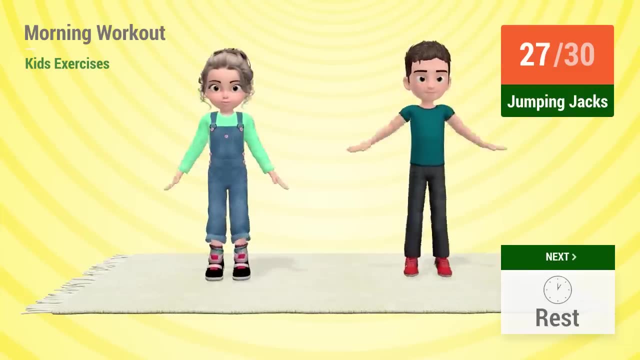 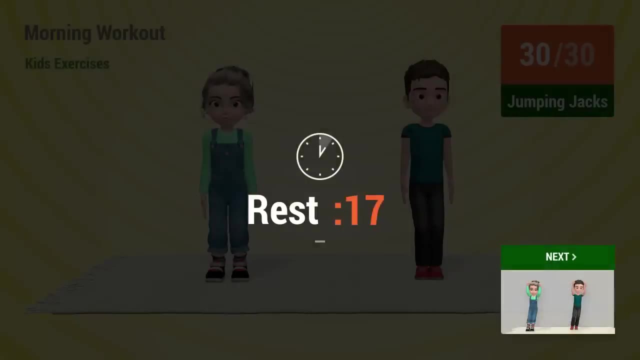 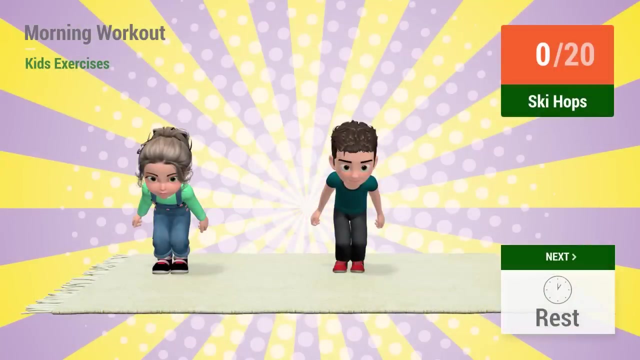 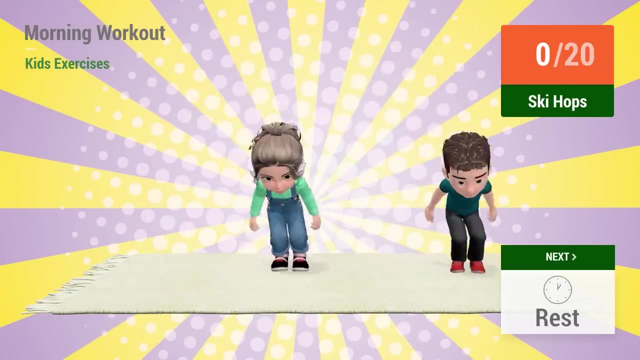 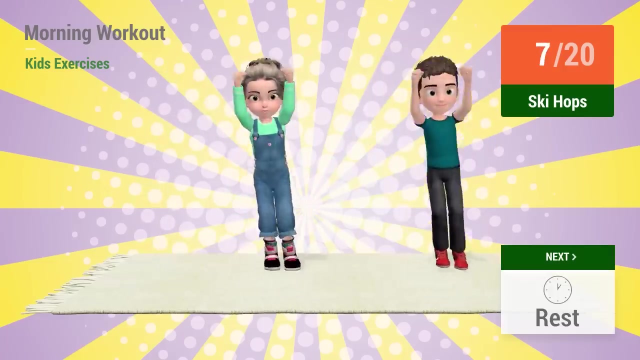 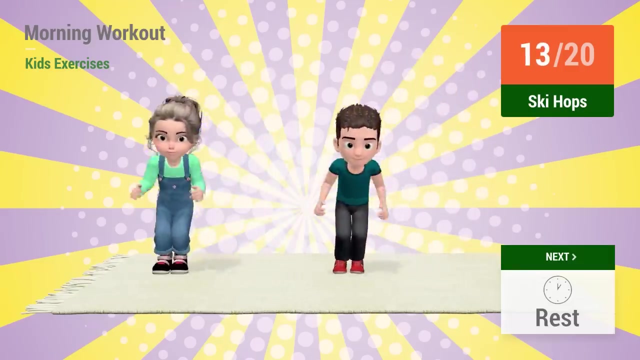 passed the three-minute mark. Keep working out. Let's see how far you can go: 22,, 23,, 24,, 25,, 26,, 27,, 28,, 29,, 30.. Rest time: Up next ski hops in 5, 4,, 3,, 2, 1, go 1, 2, 3,, 4,, 5,, 6,, 7,, 8,, 9,, 10,, 11,, 12,, 13,, 14,, 15, 16.. 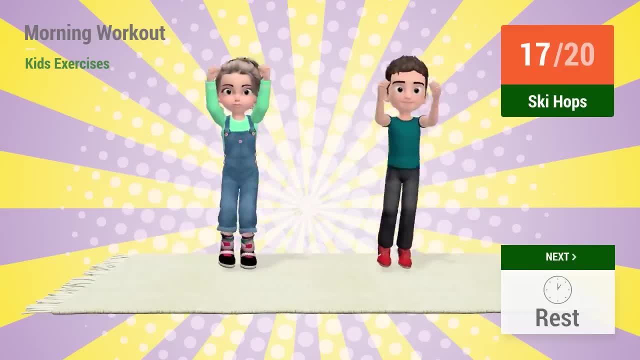 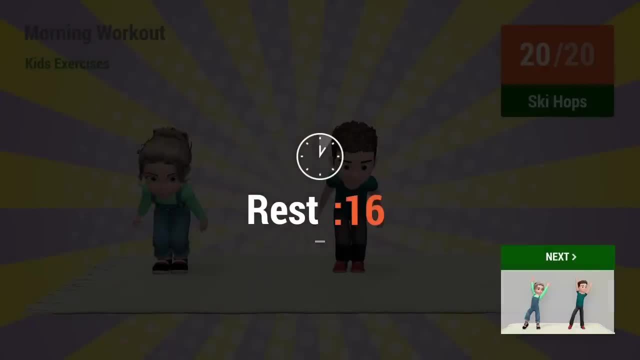 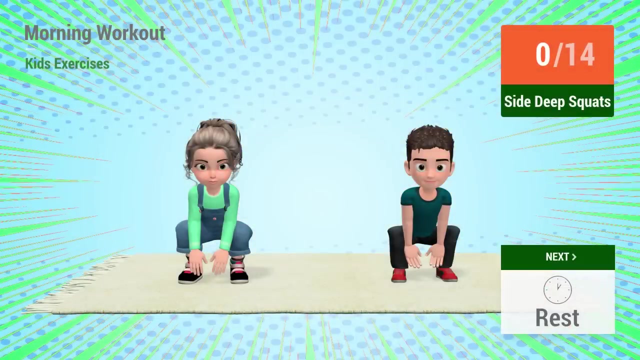 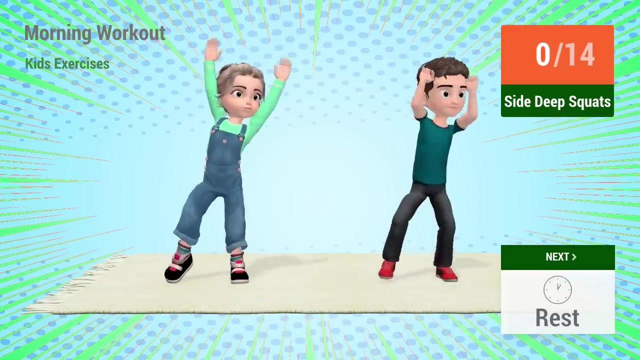 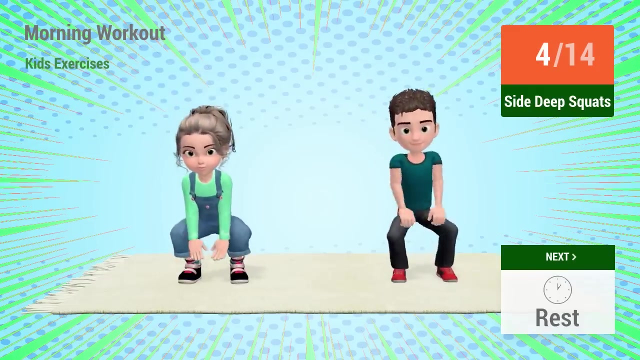 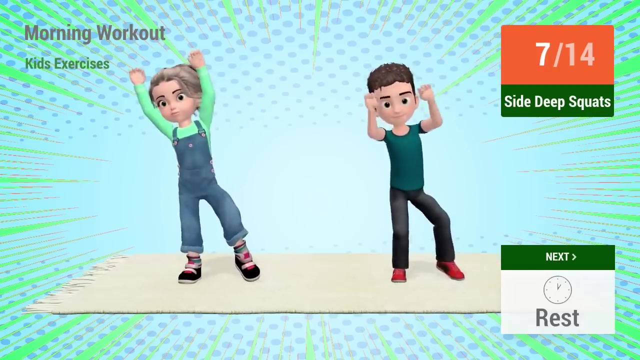 15,, 16,, 17,, 18,, 19, 20.. Rest time: Up next side deep squats in 5,, 4,, 3,, 2, 1, go 1,, 2,, 3,, 4,, 5,, 6,, 7,, 8,, 9,, 10,, 11,, 12,, 13,, 14,, 15,, 16.. 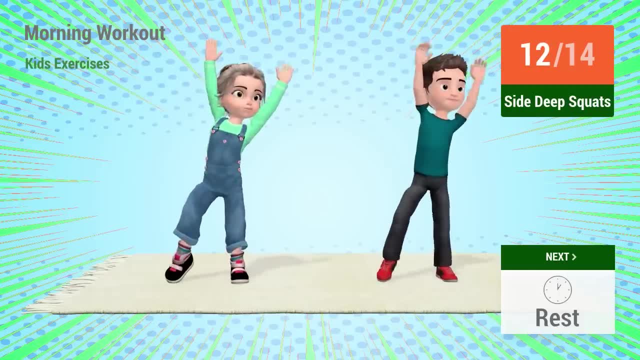 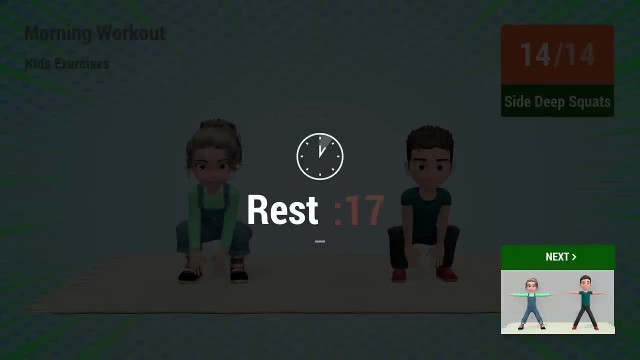 Rest time: 12,, 13,, 14,, 15,, 16,, 17,, 18,, 19,, 20.. Up next, The windmill: 12,, 13,, 14,, 15,, 16,, 17,, 18,, 19,, 20.. Rest time. 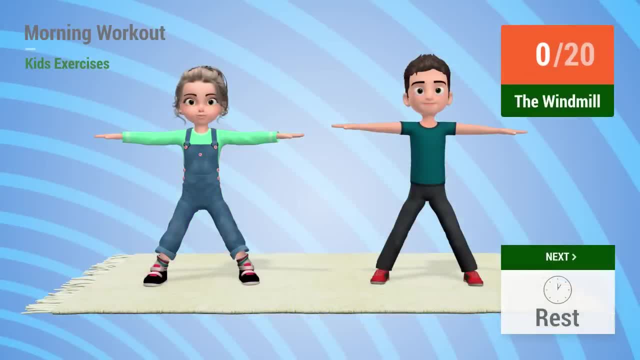 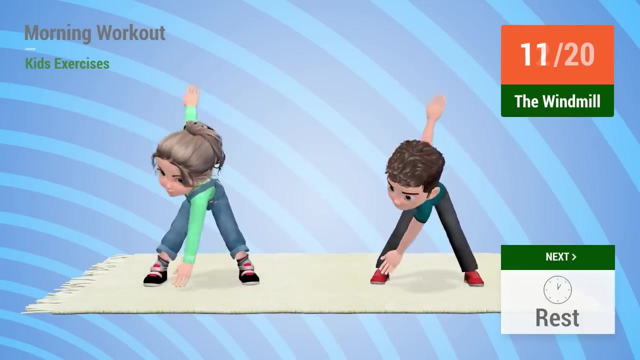 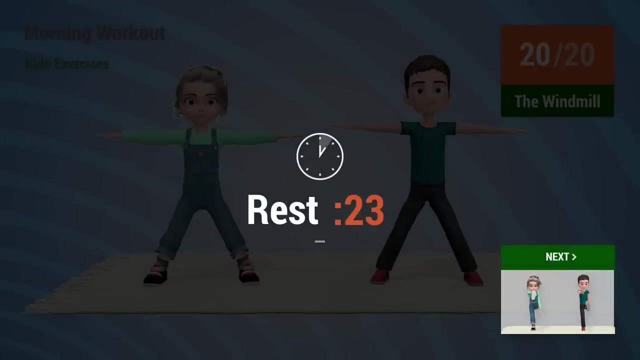 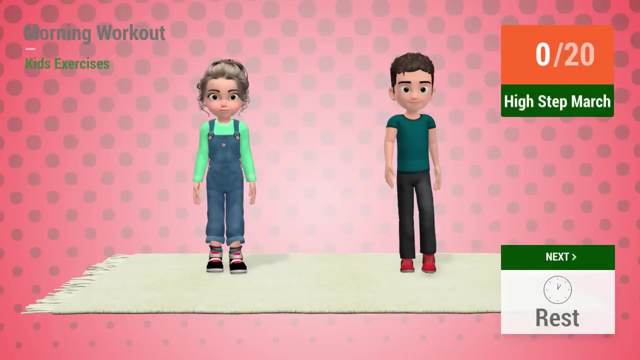 Up next in five, four, three, two, one go. one, two, three, four, five, six, seven, eight, nine, ten, 11, 12, 13, 14, 15, 16, 17, 18, 19, 20 rest time: up next high step: march in five, four, three, two, one go. 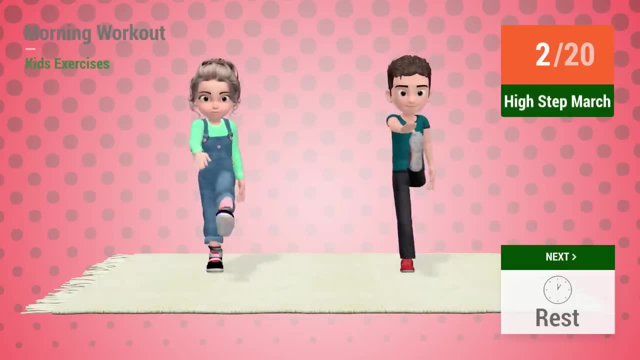 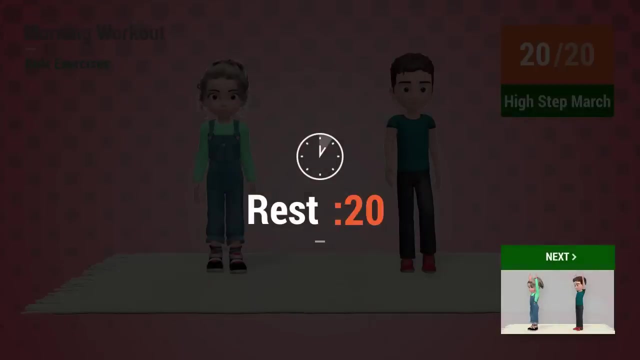 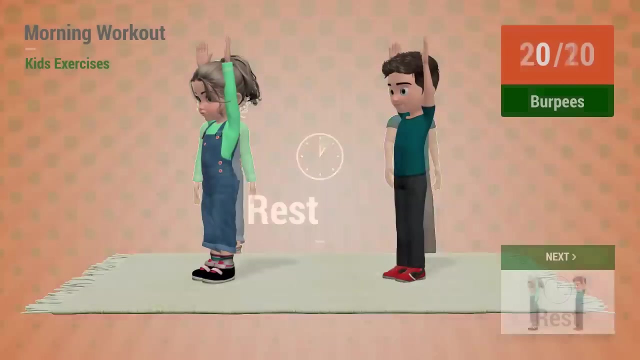 one, two, three, four, five, six, seven, eight, nine, ten, 11, 12, 13, 14, 15, 16, 17, 18, 19, 20 rest time up next high step: march in five, four, three, two, one go. 11. Spencer run up next high step: march in five, four, three, two, one go. 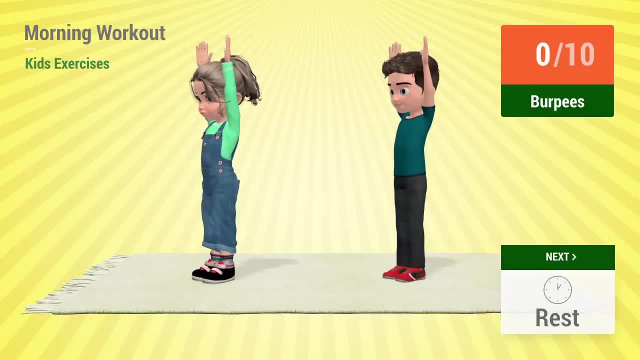 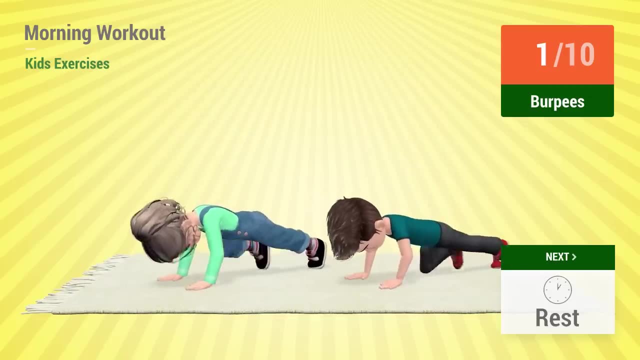 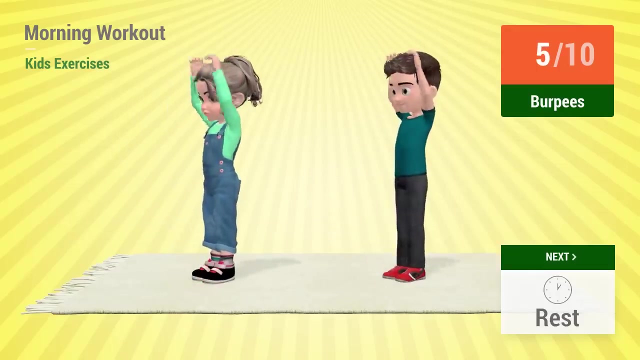 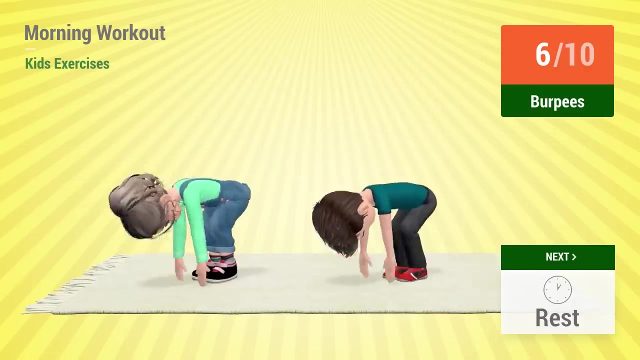 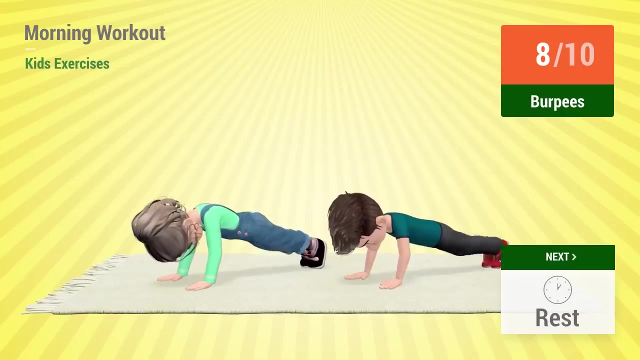 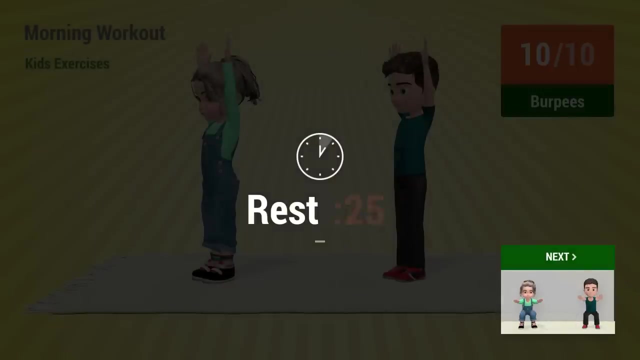 1 and 1. 3 Addition assed: 2 and 1: ı 1,, 2,, 3,, 4, 5, 6,, 7,, 8,, 9, 10.. 9, 10, rest time. 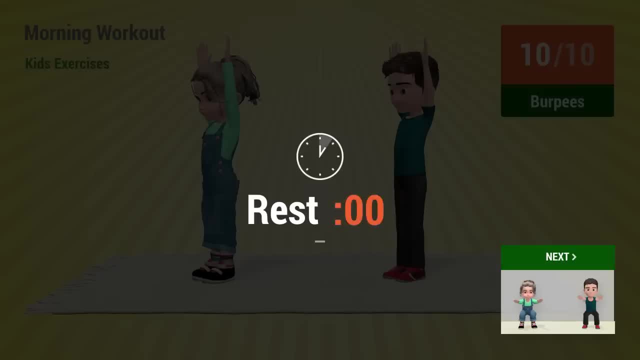 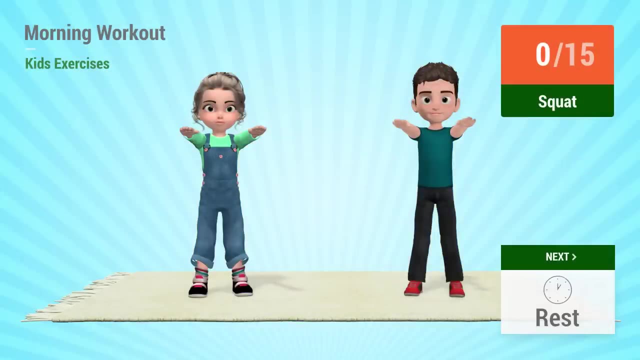 10,, 11,, 12,, 13,, 14,, 15,, 16,, 17,, 18,, 19,, 20.. 5,, 6,, 7,, 8,, 9,, 10,, 11,, 12,. 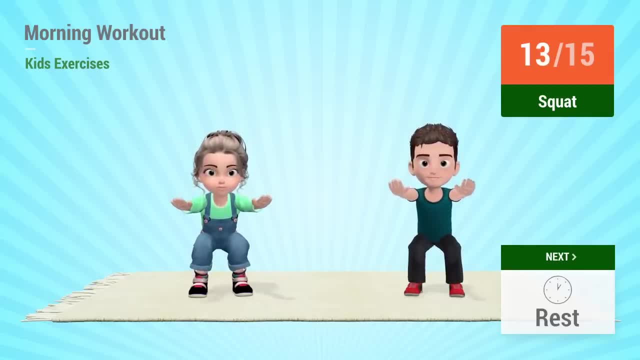 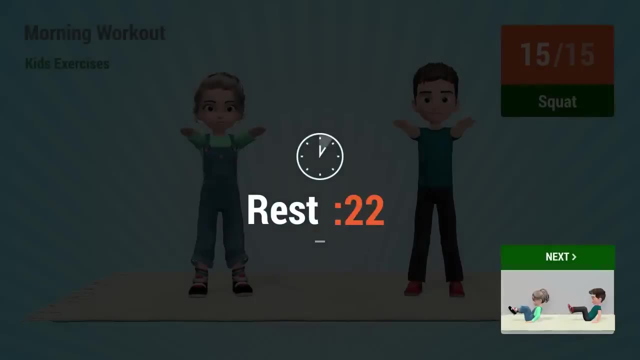 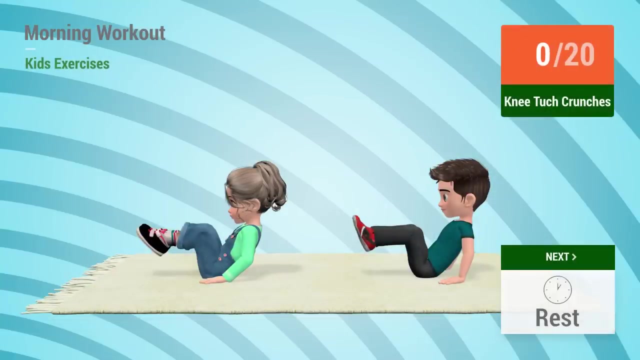 13,, 14,, 15, rest time. Up next knee, tuck crunches in 5,, 4,, 3,, 2, 1, go 1,, 2,, 3,, 4,, 5.. 6,, 7,, 8,, 9,, 10,, 11,, 12,, 13,, 14,, 15,, 16,, 17,, 18,, 19, 20.. 10,, 11,, 12,, 13,, 14,, 15,, 16,, 17,, 18,, 19,, 20.. 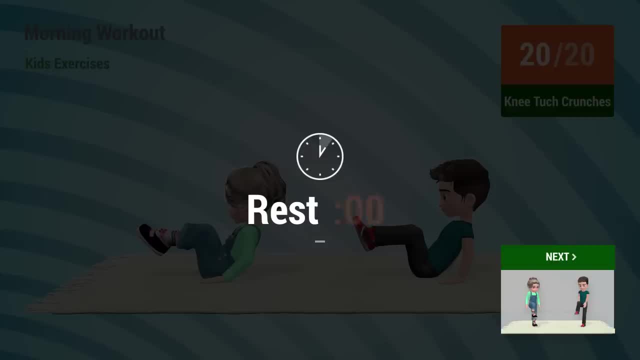 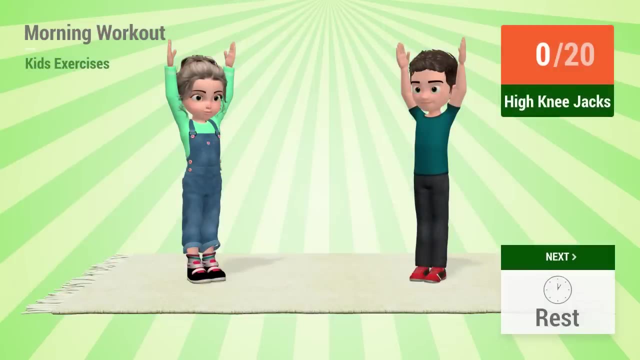 10, 12,, 13,, 14,, 5,, 6,, 7,, 8,, 9,, 10,, 11,, 12,, 13,, 18, 20.. Rest time up next: high knee jacks in 5, 4, 3, 2. 1. go 1. 2, 3, 4, 5, 6, 7, 8, 9, 10, 11, 12, 13, 14, 15. 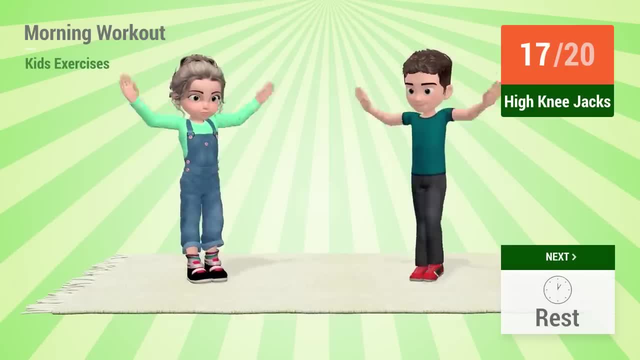 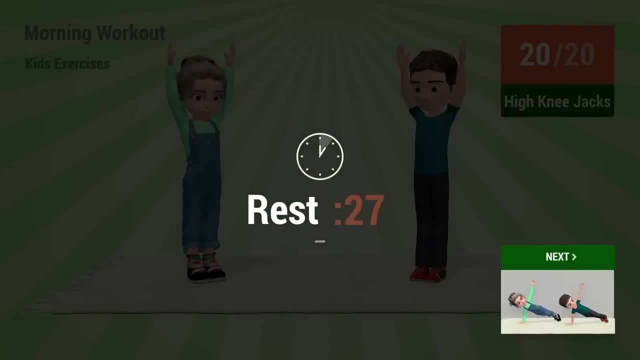 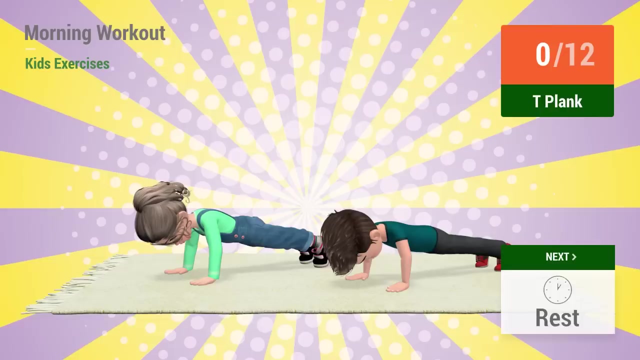 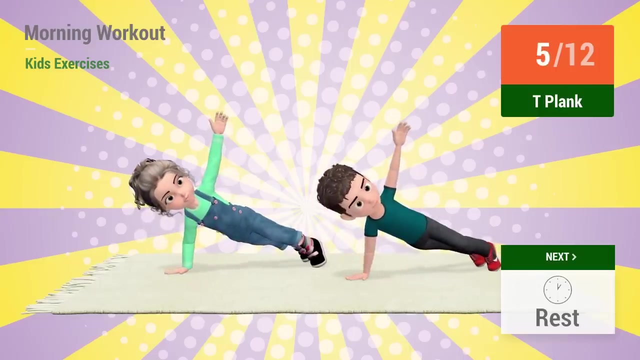 16, 17, 18, 19, 20 rest time. up next t-plank in 5, 4, 3, 2. 1 go 1, 2, 3, 4, 5, 6, 7, 8, 9, 10, 11, 12 rest time. 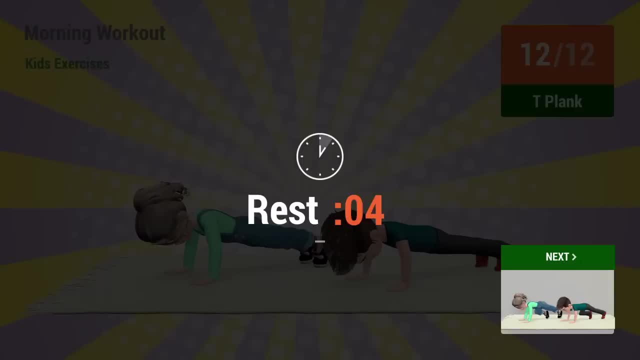 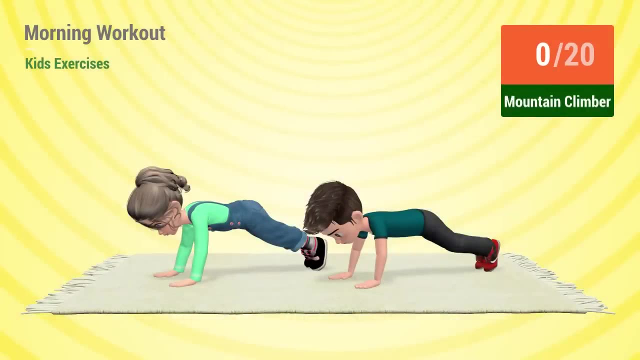 up next mountain climber in 5, 4, 3, 2, 1 go 1, 2, 3, 4, 5, 6, 7, 8, 9, 10, 10, 11, 12, 13, 14, 15, 16, 17, 18, 19, 20.